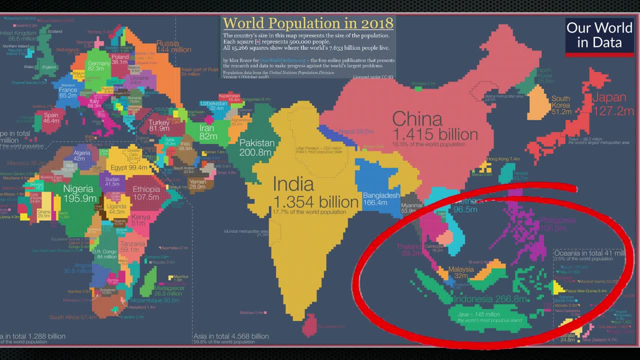 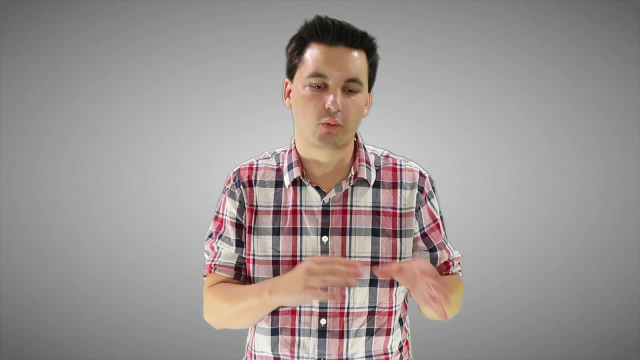 ourselves. The last region is in Southeast Asia, And here we're looking at countries like the Philippines, thailand, where their populations have been booming in recent decades. now we've been talking about different regions around the world, but if we change our scale to a more local scale, we can. 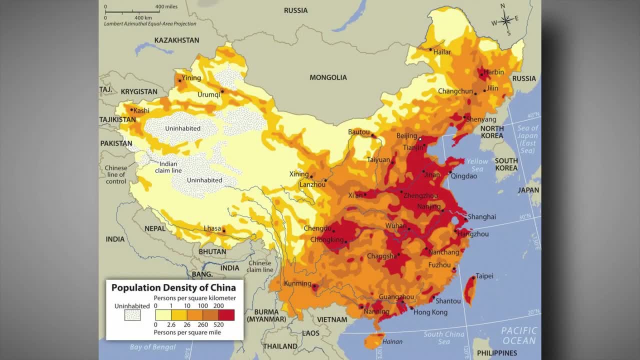 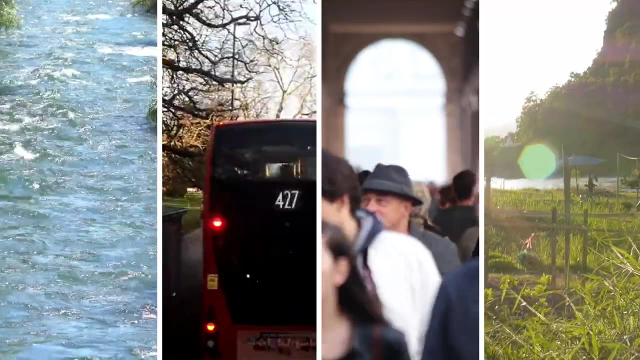 actually start to see some trends that are occurring in all these different regions. when looking at this population density map of china, notice how the areas with the highest population density are near the coastlines and rivers. this isn't by chance. when we look at different population clusters around the world, we can see common themes. site and situation factors have a 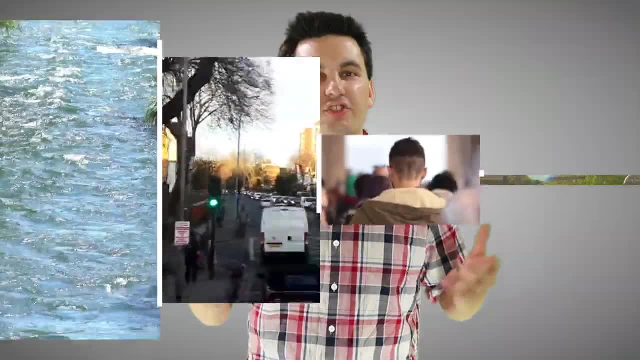 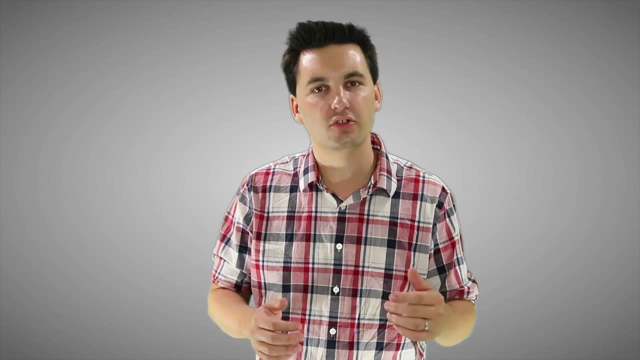 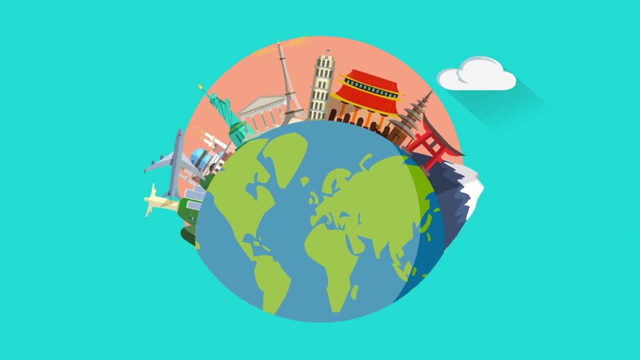 huge impact on the location of settlement. remember, site factors have to do with the location itself- it's dealing with physical features, while situation factors are dealing with factors that exist in the surrounding area. when looking at major settlements around the world, we can see that many of them center around fresh water, a river, an ocean, fertile soil. this is because they need food. 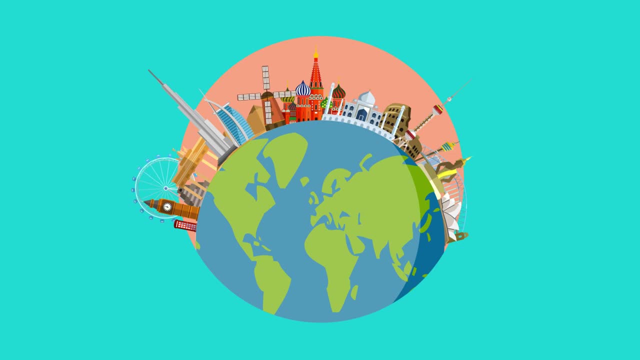 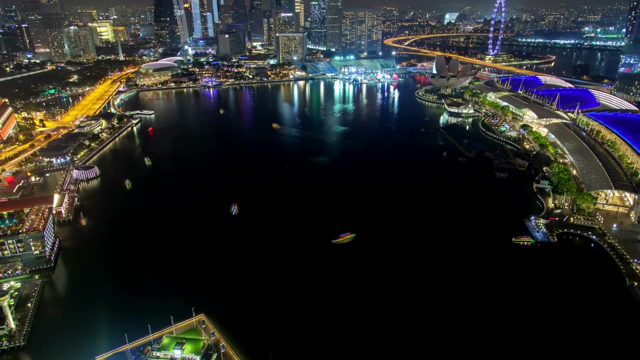 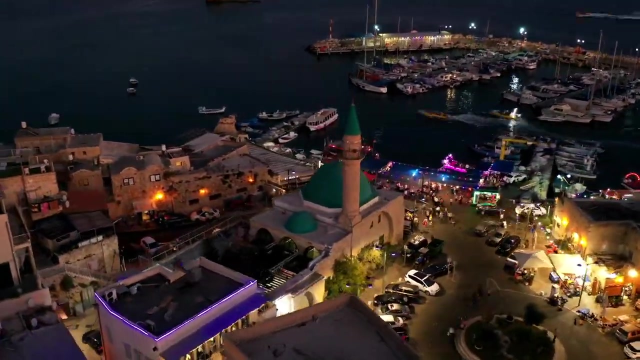 and water to survive, and the reason why we see many of these settlements on coastlines or by an ocean or river is because they want to trade. they want access to the water so they can connect with other settlements in different geographic areas. now, it's not just food and water on why we live in certain areas, it's 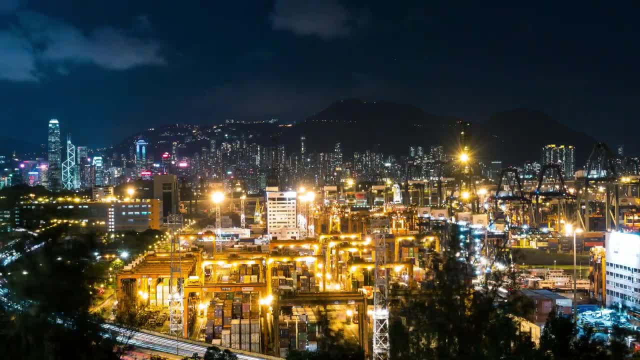 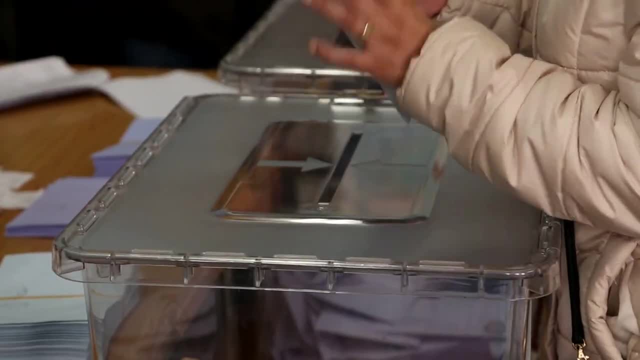 also because of economic reasons. we want to live in an area that actually has a job for us and where we can advance in our careers. or maybe we're living in an area because of its political stability- we feel safe there and secure. or it could be because of the fact that we live in a 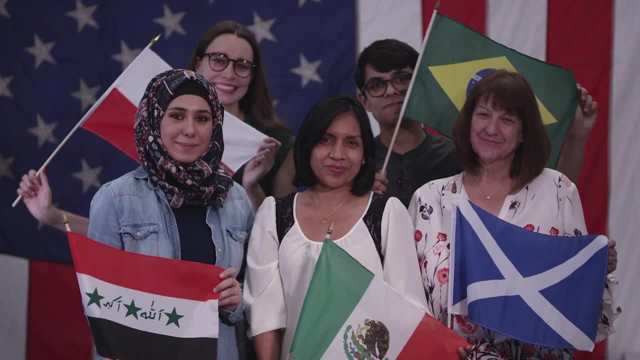 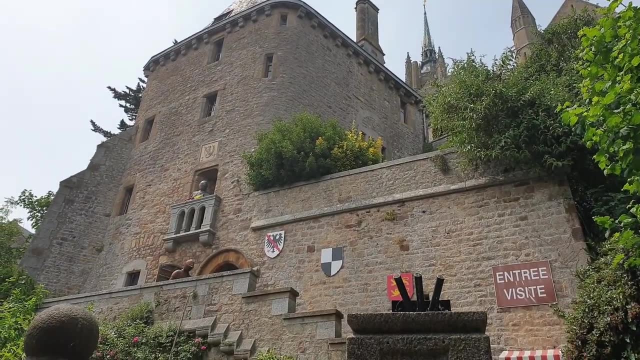 place where we have a lot of cultural preferences. we can see ourselves in the community and we feel a part of our settlement, our city, our society, and sometimes it's even just because of the historical events that created the settlement in the first place. we can also look at areas around the world. 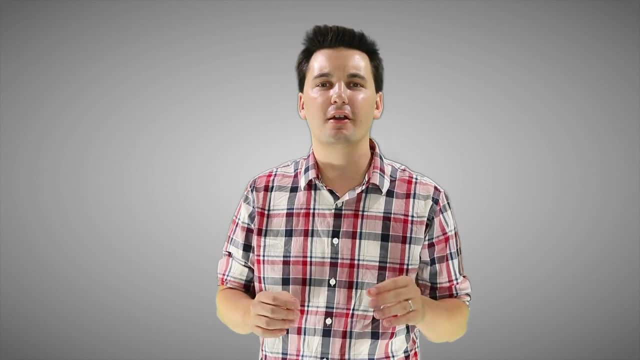 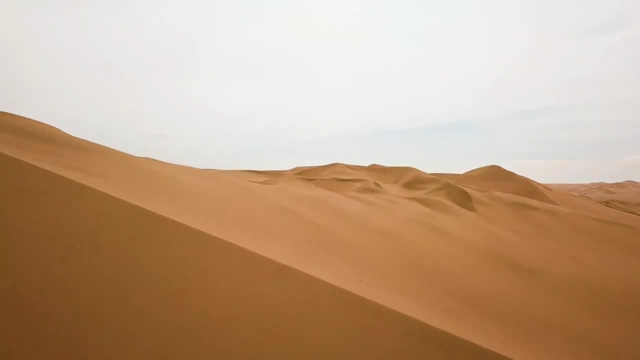 where we actually can see people don't really want to live. these are areas that are kind of, too, they're too dry, they're too wet, they're too cold or they're too high. places that are too dry, well, it's difficult to be able to produce crops and to be able to have a stable society. places that 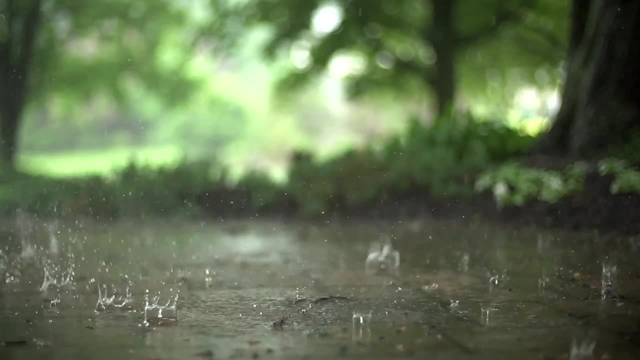 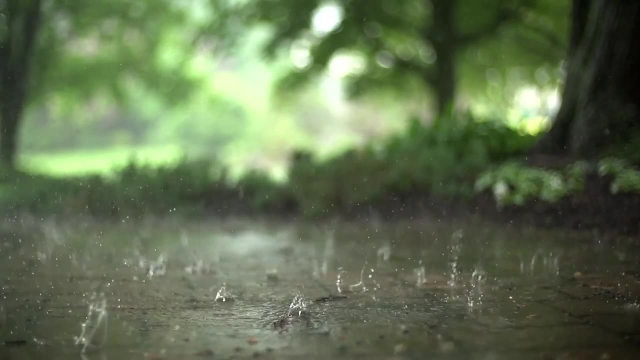 have a similar problem. if it's raining too much, our soil might become oversaturated, and especially if we mix that with humidity and heat, we actually might see the nutrients get pulled out of the soil, making it more difficult to have sedentary agriculture and places that are too cold and 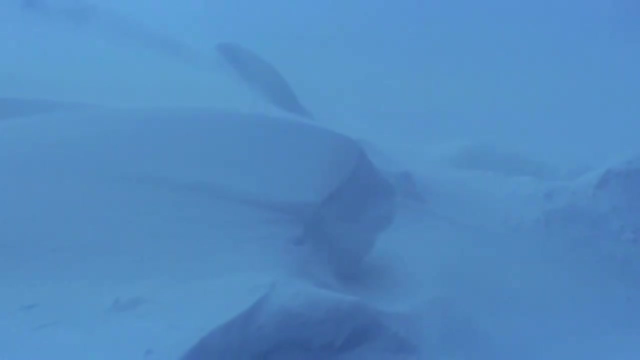 too high. well, just, it's hard to be able to get all the resources that we need to be able to survive and to also be able to have a high standard of living. people don't want to live in areas where you're going to struggle to survive, especially in the modern era, but at the same time, we're now. 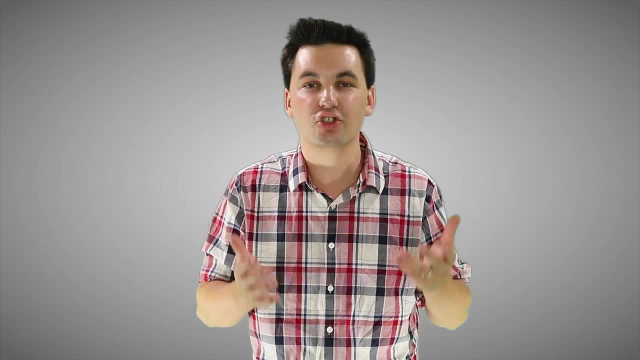 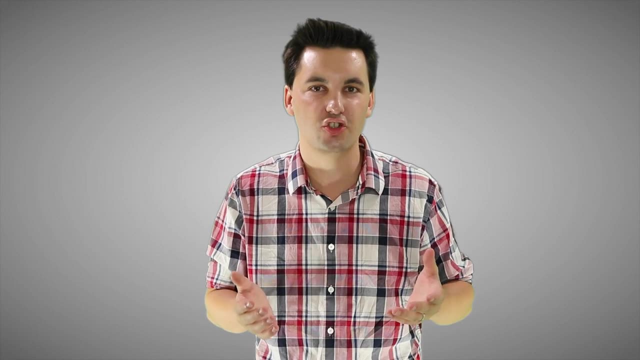 going to be able to live in areas where settlements develop, in geographic areas where before it just wasn't possible to have sustainable societies there. now we're seeing this. because of advancements in technology and communication, we're now able to modify our environment to make it hospitable. 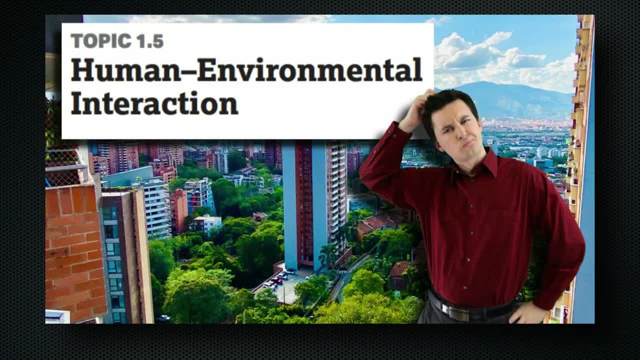 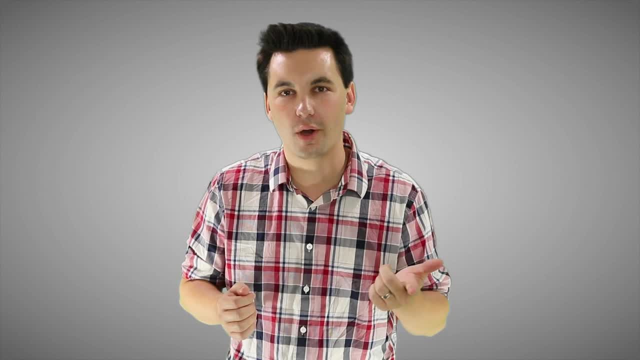 and this is connecting back to a concept we talked about in unit one, topic five: environmental possibleism. if you need more information on that, go check out that video. okay, so so far we've been talking about where people are living in the world, why they want to live in certain areas and also. 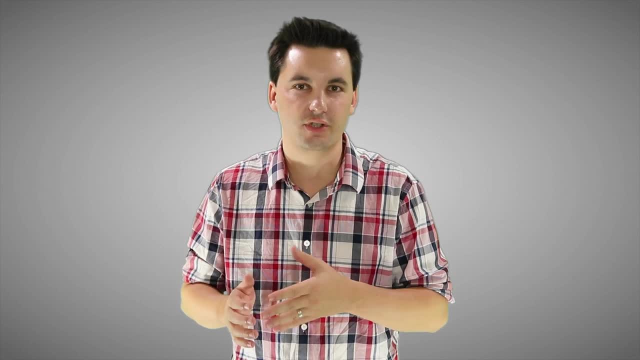 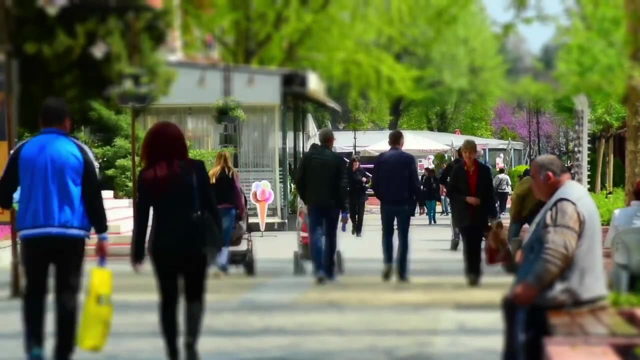 why they don't want to live in certain areas of the world. now we're going to be getting into population density more. we've mentioned population density already in this video. population density is just looking at how many people are living in a certain geographic area and we can see population density broken into three different density: the 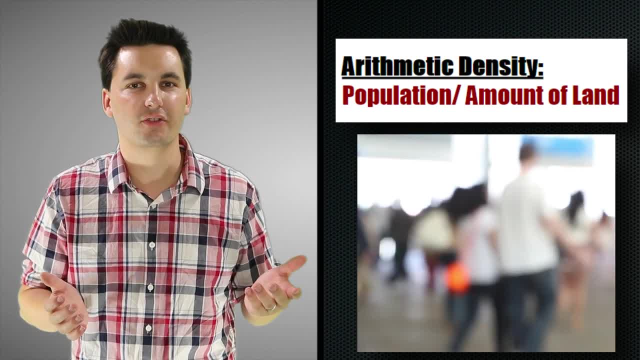 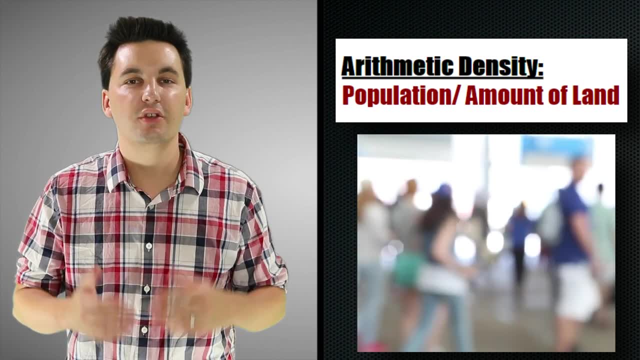 first density is our easiest density defined. it's our arithmetic density. this density would be calculated by taking the total population and dividing it by the total amount of land. this density shows us just how spread out people are. if this number is really high, it probably means that 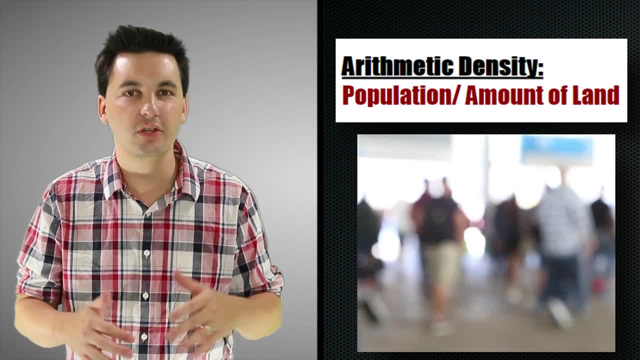 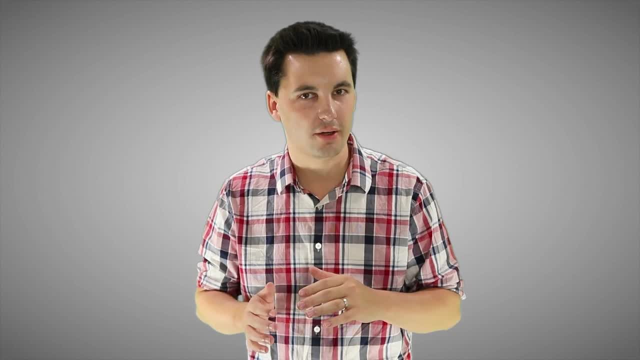 people are clustered together. on the other hand, if it's really low, it means they're probably dispersed throughout society. now one thing to think about: when we're looking at this density, remember we're dividing it by total land. that means there could be land in here that no one's 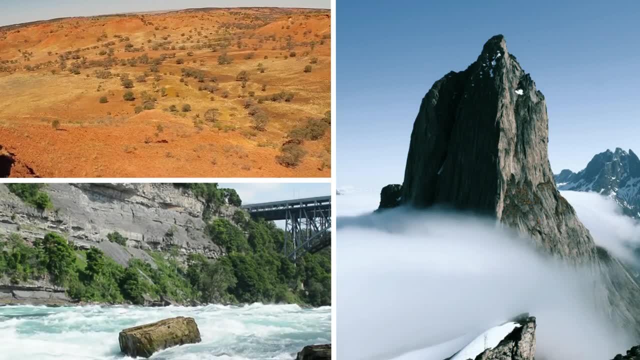 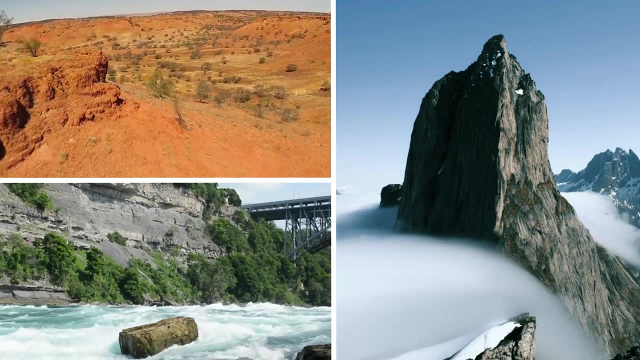 living on. maybe it's a mountain range, maybe it's just not fertile soil and people don't have a desire to live there, or it's a river. there's a variety of factors that could be at play here, so this could create some distortion in our numbers, and we just have to take that into account. 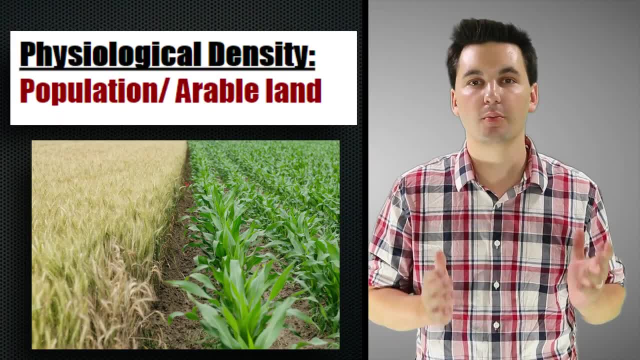 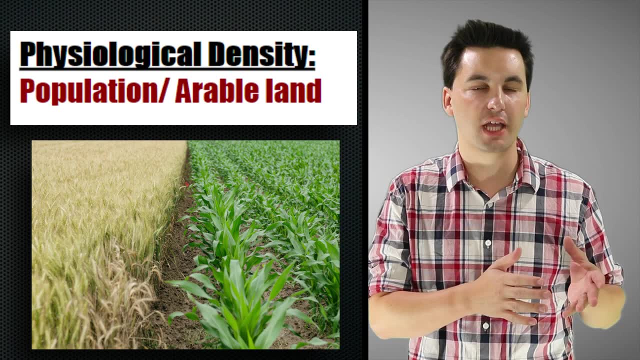 the next density is our physiological density, and this one's really important because we're gonna be really important. We can actually gain more insight into society by looking at this one To find it. what we're going to do is take our total population again, but this time we're going. 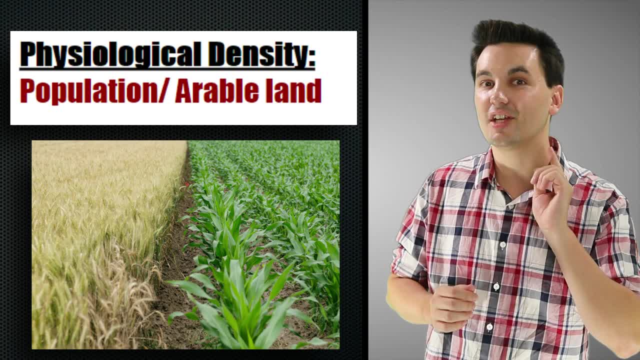 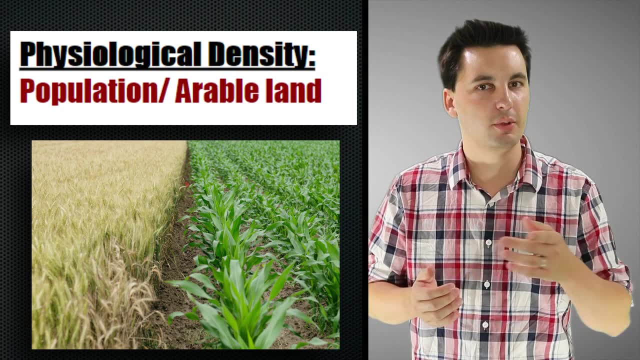 to divide it by our total amount of arable land. Notice, I said total amount of arable land. This is land that can produce food. What this density will really show us is how much stress are we going to be putting on each unit of land. The higher this density number is, that means we need 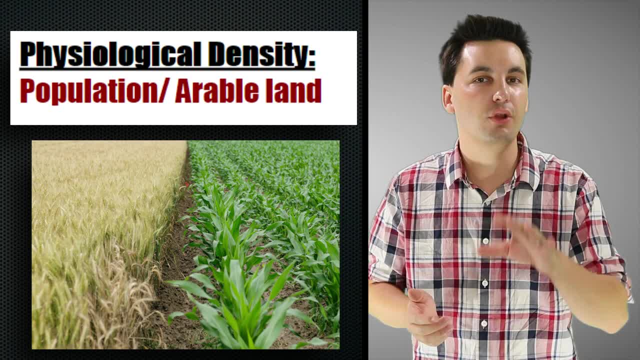 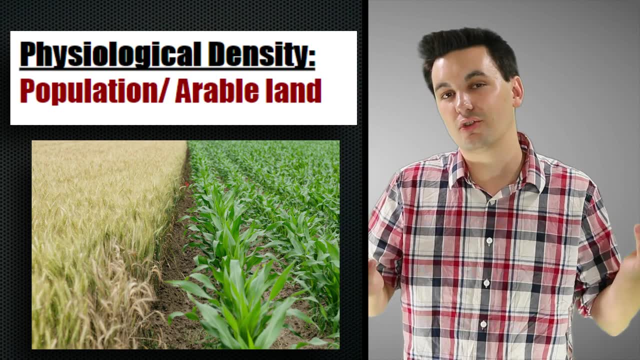 to be able to get more food out of just one section of land. The lower it is, the less stress will be put on our land, because we'll have to produce less food for each unit of land. This means that if it's a lower number, we're probably going to be able to protect our natural resources better. 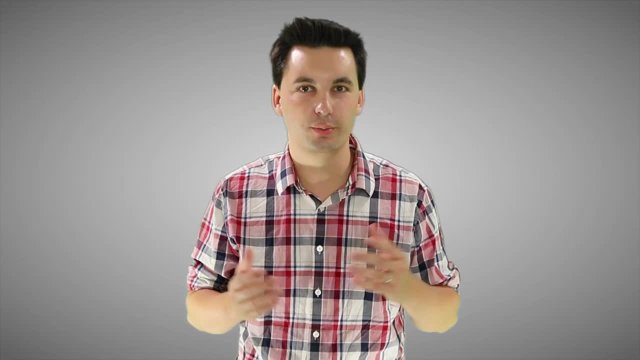 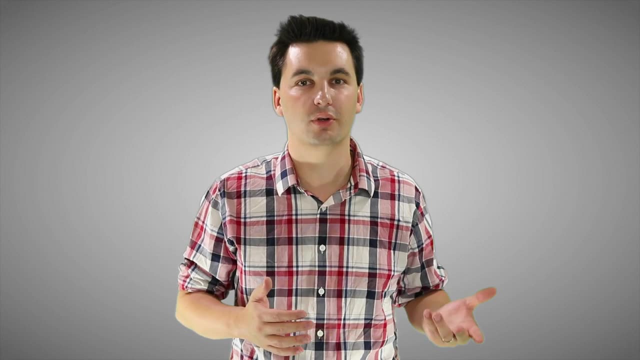 by not overusing them, And if it's a higher number, we might be at risk of depleting our nutrients that are in the soil and we might see desertification occur, and that could force us to rely to get food from other countries. So we would have to focus more on trade instead of producing. 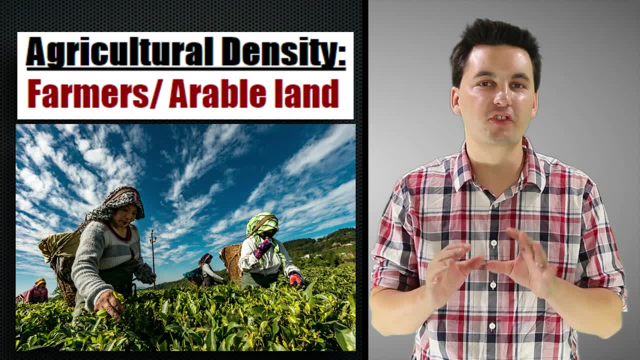 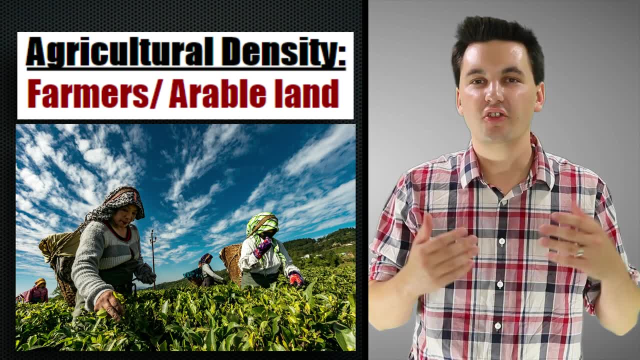 it ourselves. The last density is our agricultural density, and this density, we're going to take the total amount of farmers and we're going to divide it by the total amount of arable land. What this density shows us is how efficient is agriculture in our society, How much technology are 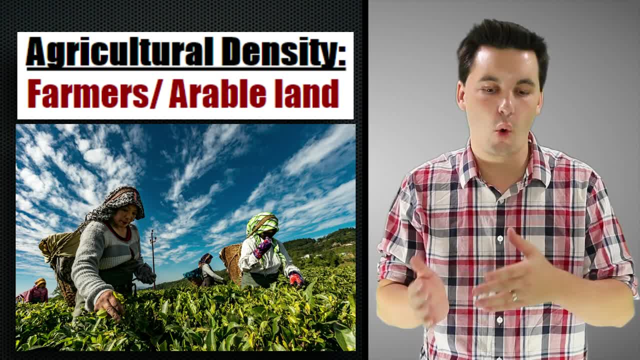 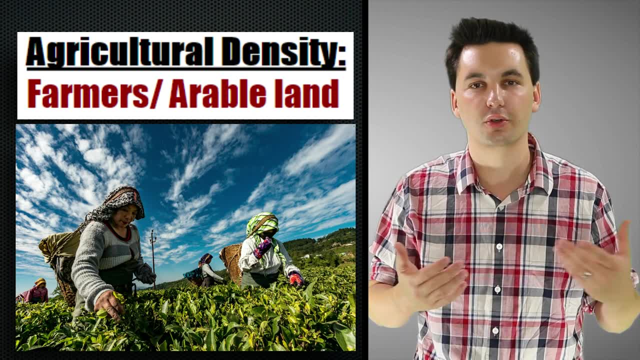 we using The higher this number. well, that means we're using more human labor to be able to produce food. The lower the number, the less amount of people are needed in order to be able to produce our food. If this is a lower number, it means that we could have people specialize in other areas of 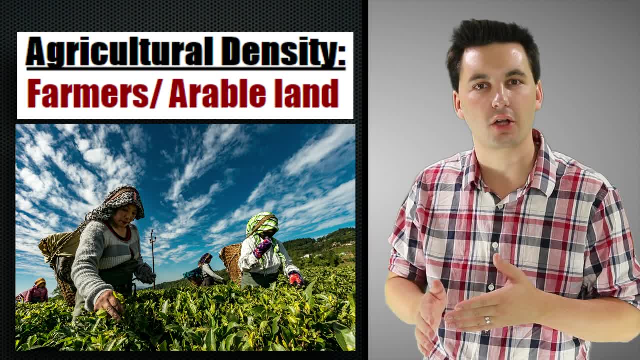 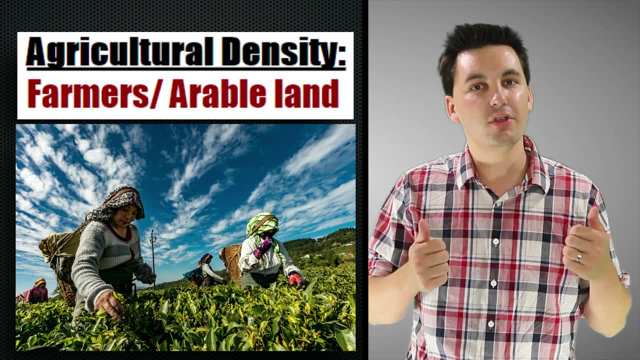 the economy and we don't need to have so many people focused on agriculture. Normally, this shows that the economy is more efficient. as they'll start to see, then, other sectors of the economy take off. The higher the number is, well, that means it's less efficient. We have to have more people. 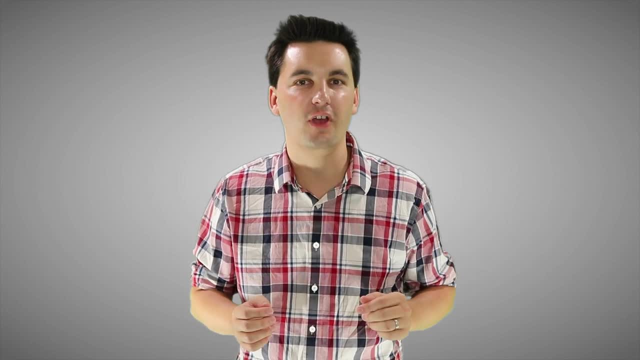 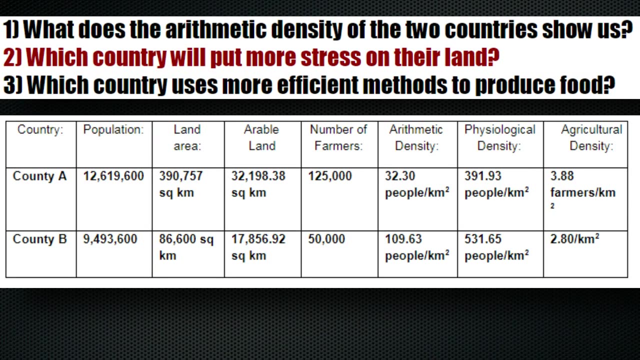 doing the same task. These densities by themselves are important and they show different aspects of society, but the real insight comes when we compare and contrast them and we look at them as a whole. Take a second actually right now. Look, we have country A and B. What inferences can you make about? 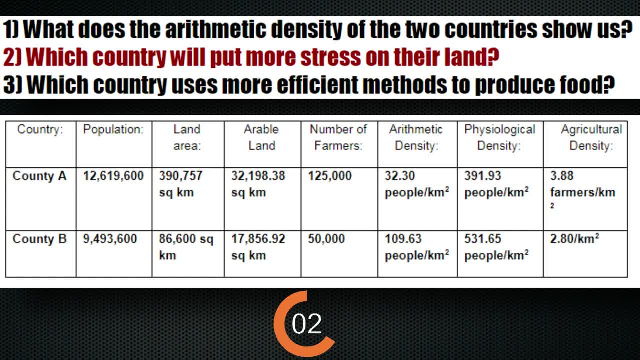